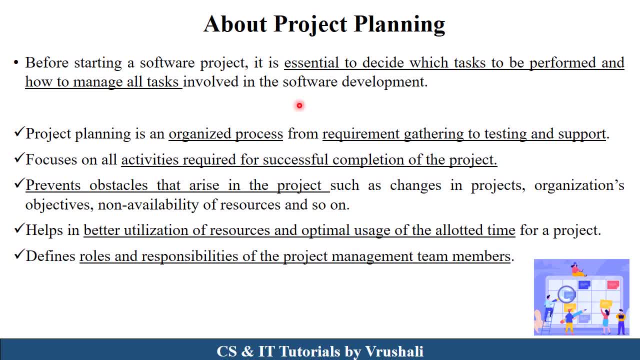 project planning: See as per the software development life cycle. after requirement gathering and analysis, The next phase is planning phase. After planning, designing, development, testing, these phases have occurred. Project planning is one of the most important phase because they decide. 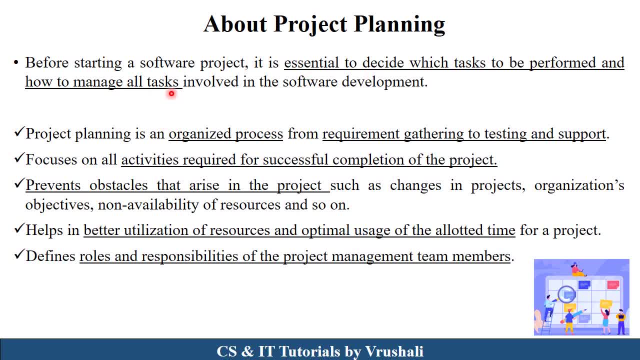 which task to be performed and how to manage all tasks in SDLC phases. As per the definition, project planning is an organized process because they handle all the process that have occurred in between requirement gathering, analysis, then designing, development, testing and, after that, deployment and maintenance phase. Basically, they handle all the activities. 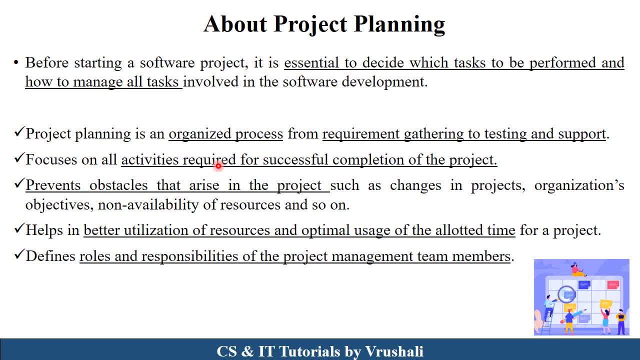 that will be useful for successful completion of project. In software project there are some issues or obstacles have occurred, like changing project requirement, then the organization objectives, then non-availability of resources, right. So these all types of obstacles also prevent and solve in project planning phase. Basically, project planning helps in. basically 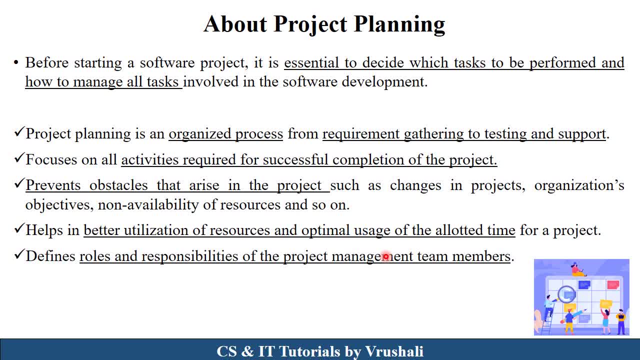 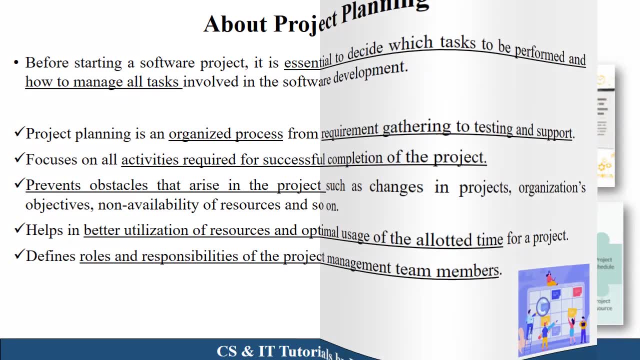 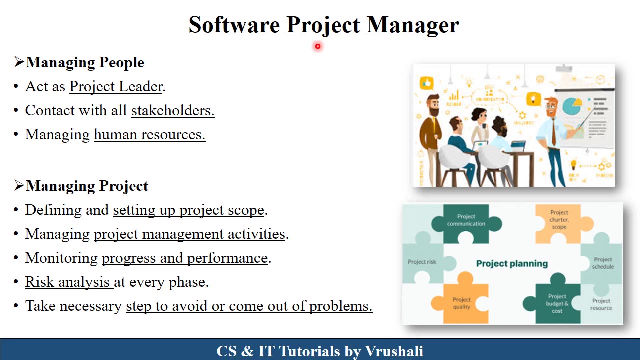 better utilization of resources and completing your project in proper allotted time. Project planning phase also defined roles and responsibility of each and every person that involved in particular project. That's why project planning is an important phase. Now, what exactly software project manager? So software project manager is a person who 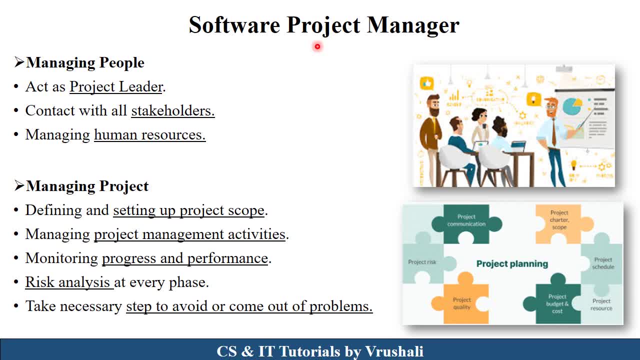 handle this complete project planning phase. Basically, they manage people and also manage the company and the team. So these are the things which you have to be preferred by the manage project. so software project manager act as a project leader. they contact with all the stakeholder. they also contact with all the customers. they 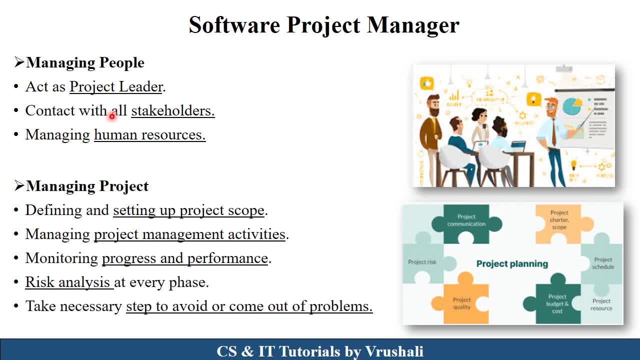 identify their needs, requirements and also issues that customers have occurred. basically, they manage all the human resources. the software project manager also define a complete project scope. then which type of project management activities are there? they also monitor complete progress and performance of project. they also find out risk analysis at every phase and basically, 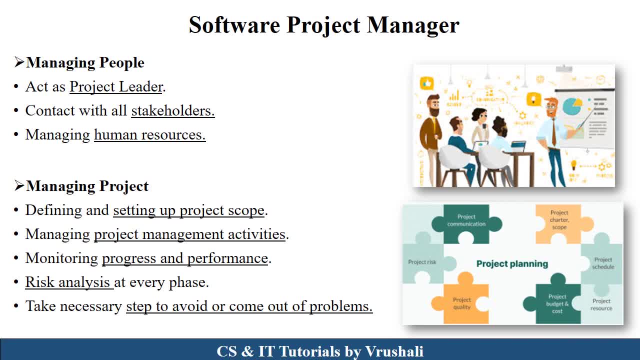 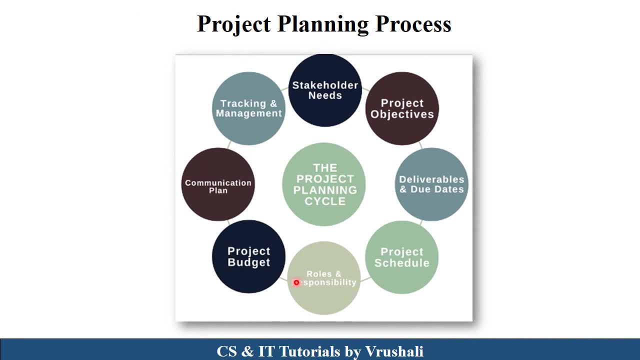 they also avoid. all types of problems have occurred in each and every software development lifecycle phase. so basically this project planning phase are handled by software project manager. now the next topic is project planning process. so basically there are total eight step in project planning process. let discuss all. 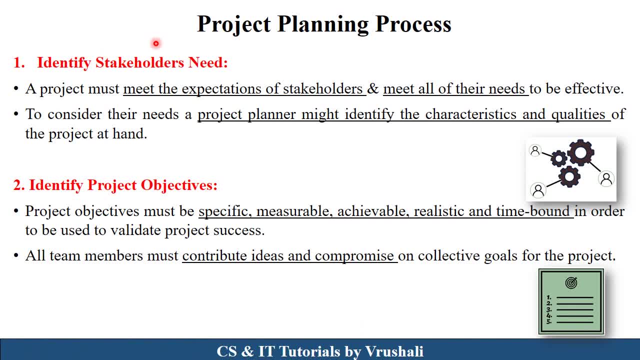 the steps in detail. the first step in project planning process is identify stakeholders need see. basically the most important is customer: what exactly customer want. this is the first priority of any project head right. so in the first process you must know what exactly customer want. what is the need of the customer? so to identify all those 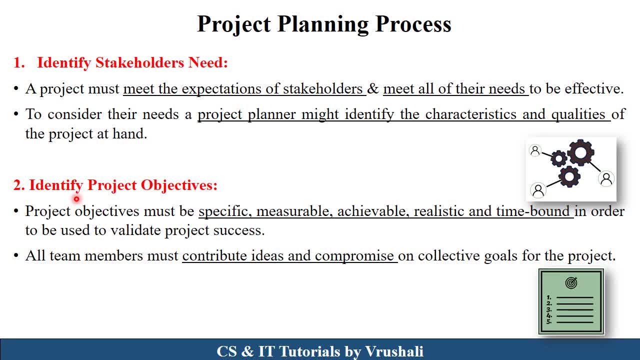 thing. this is the first step. now, in second step, identify project objective so as discuss with customer what exactly customer want, what is objective in goal of the customer? to identify those thing. this is called a project objectives. so this project objectives must be specific, measurable, achievable, realistic and time-bound in 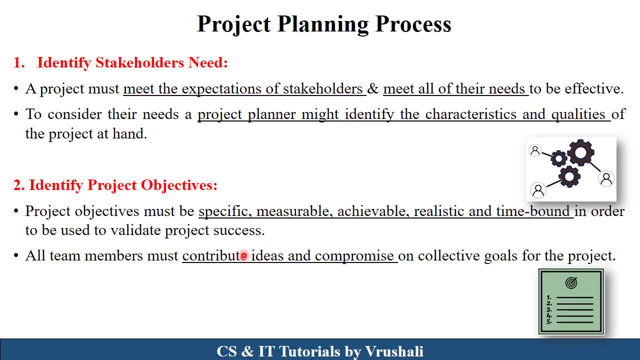 order to validate a project. success means this project objectives are very much important, that will be easy to fulfill, easy to achieve and that will be completed in particular time. and that will be measurable means there are finite requirements, not infinite requirements, right? so basically, all team members contributes their ideas and compromises also. 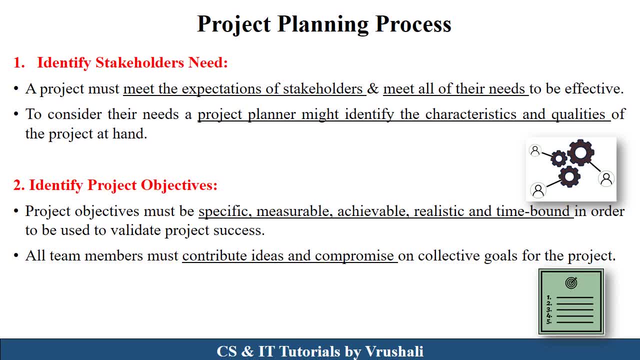 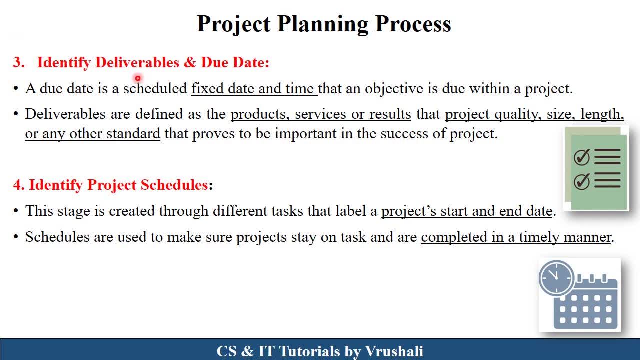 regarding particular collective goals, so this is called as project objectives. the third step is identify deliverables and due date. so deliverables means each and every functionalities included in particular project, for example, product services or results means the quality of the project, the size of the project, the length of the project and the standard of. 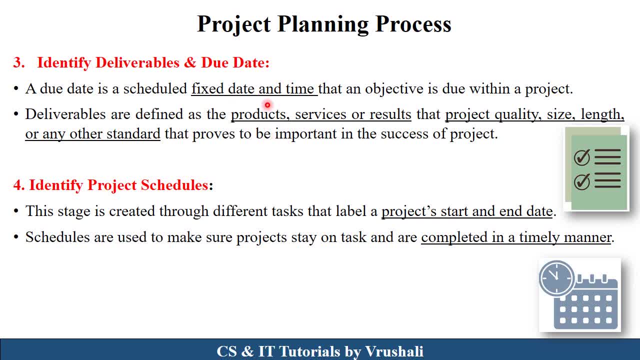 the project. so identify all those things and you have to complete each and every phase in software development lifecycle within a due date means proper time required for planning phase. after that, proper time required for designing phase. after that, particular time required for development. So every phases have completed within a due date. next step is identify project schedule. 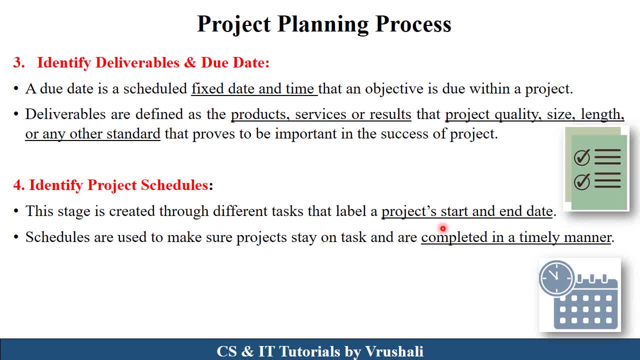 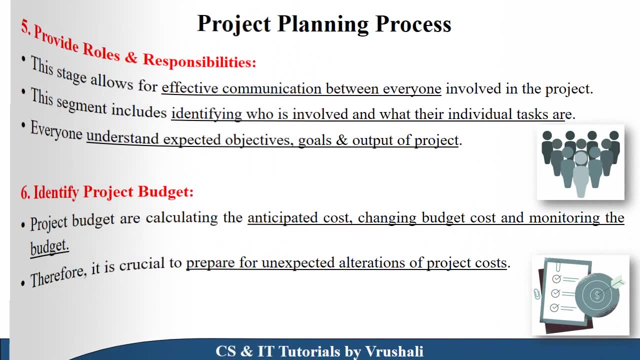 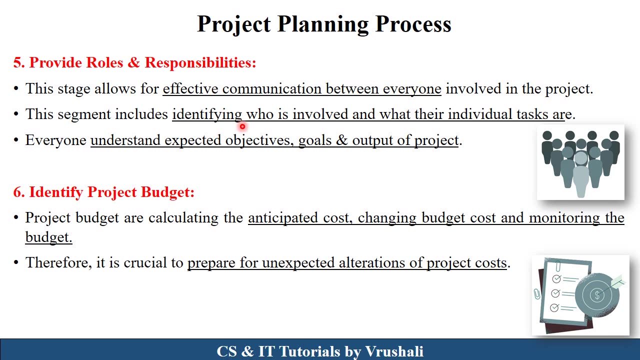 so project schedule basically means when projects will start and the end of the project means each and every task, each and every phases have completed in timely manner. so project schedule, project deadline, also have decided in project planning process. the next process is provide roles and responsibilities. So basically their are different stakeholders are included in particular project. 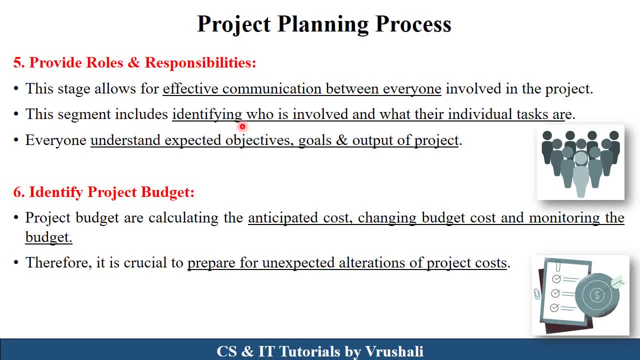 So means each and every recognise which type of roles are there, For example, designer, developer, tester day, then project manager, then our support engineer is there. So there is an effective communication between everyone. so identify roles and responsibility of each and every person. and this: all persons have performed same type of objective, same 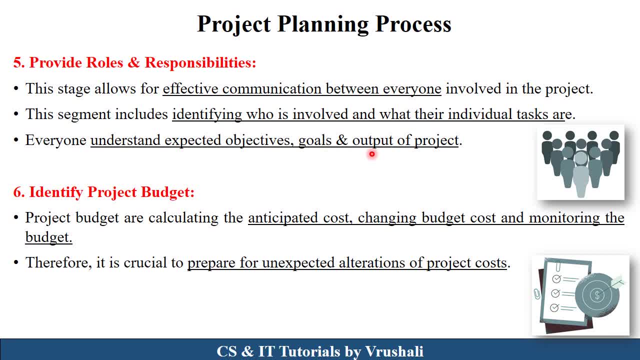 type of goal Because in this year- have fun- It generate a proper output at the end of the project as per the customer requirement. So here, project manager, provide roles and responsibilities to each and every stakeholders. The next process is identify project budget. So budget is one of the most important thing is project planning phase. 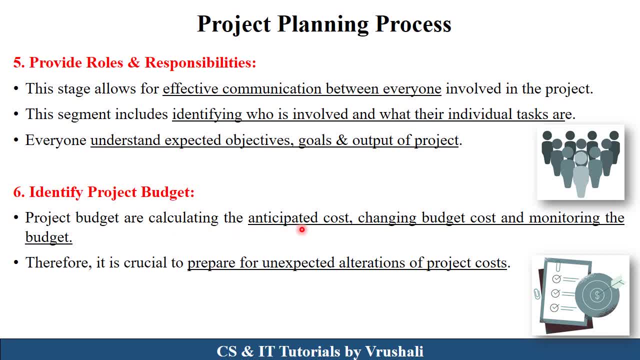 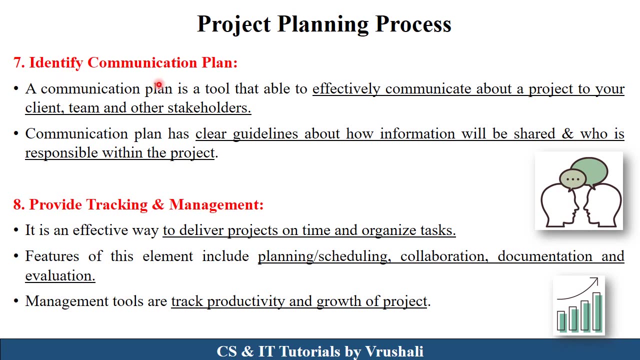 So here project manager calculated. the anticipated cost means what exactly cost required for completing the particular project. And if but customer requirements have changes, So budget and cost is also changes. So they monitor the complete budget process for particular project. The next step is identify communication plan. 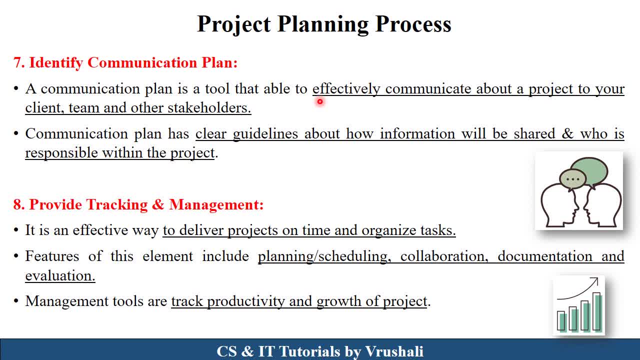 See, in software development lifecycle communication is too much important because designer design a particular product, Then they deliver this particular design to the developer team. right: developer develop the product And send forward to the tester means there is a communication required between designer, developer and tester. 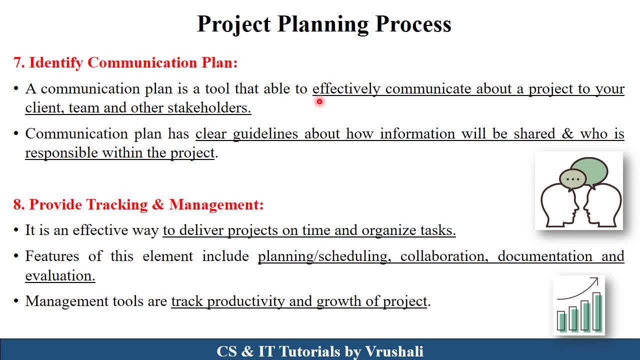 So this is a communication plan. So communication plan provide a clear guidelines about how each and every information have shared and who is responsible for particular activity and particular task. And the last step is provide tracking and management. So here, project manager, deliver a complete project on time. 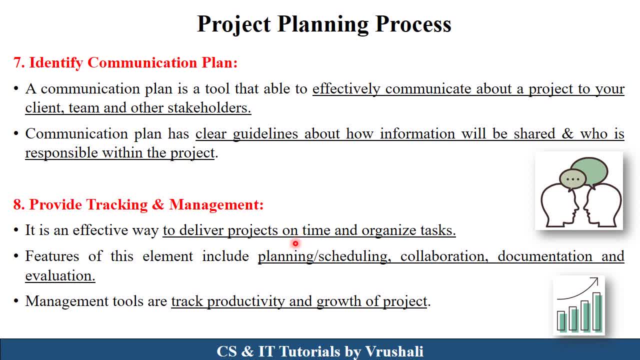 And, in particular, Organized manner. so here they track or manage complete schedule of project collaboration. documentation and evaluation of project means the track, each and every activities included in particular project, from designing to deployment phases. basically there are different management tools. they track productivity and the growth of project. means your project have completed within time within budget.